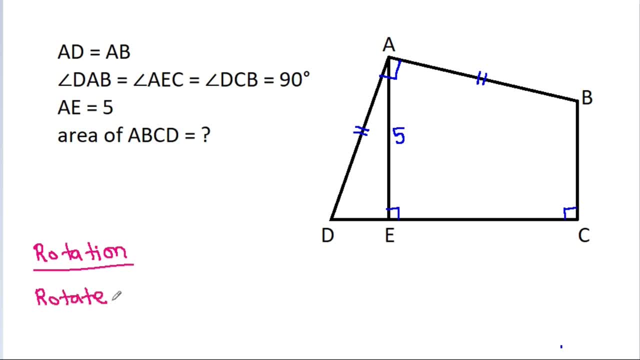 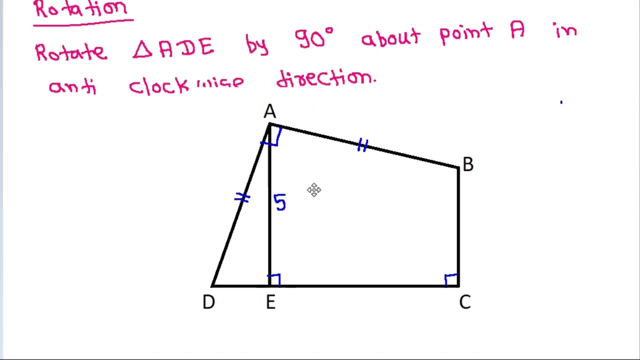 If we rotate triangle ADE by 90 degree about point A in anticanoqueous direction, Then Angon DAB is 90 degree and DA is equal to AB. So point D will come at point B. Suppose D' and DE is horizontal. 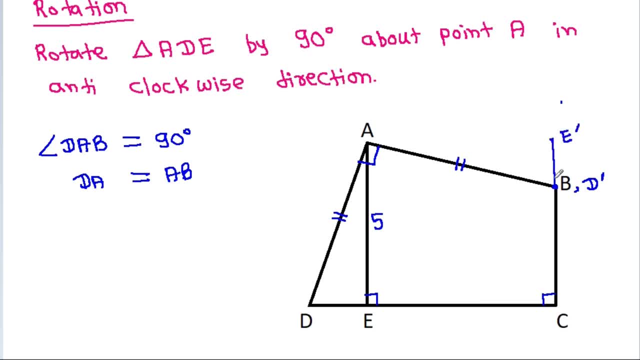 So D'E' will be vertical And these two areas will be equal And this angle will be equal to this angle. And Angon DAB is equal to 90 degree, So Angon EA will be also equal to 90 degree. 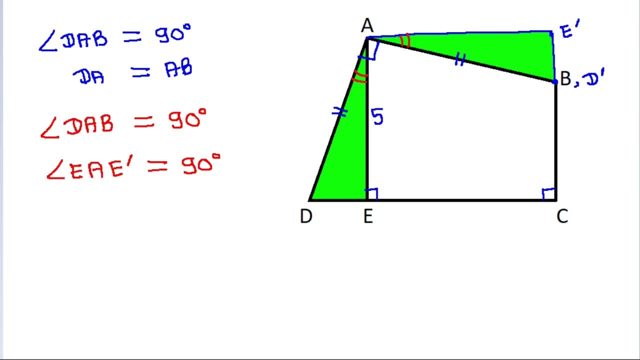 and in AEE'CE AE is 5 and AE will be equal to AEE'CE. that will be 5.. This angle is 90 degree. This angle is 100 degree. So this angle is 95 degree is 90 degree. this angle is 90 degree, so this angle will be also 90 degree. So, area of AEC.